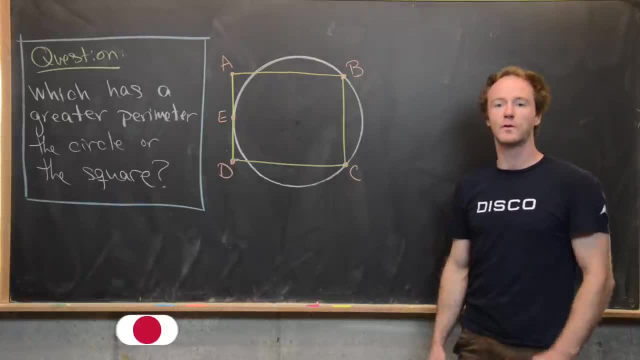 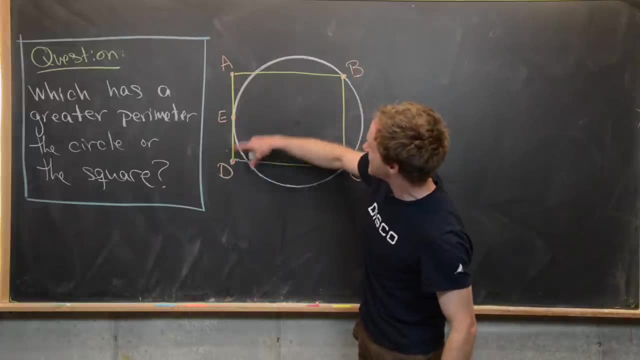 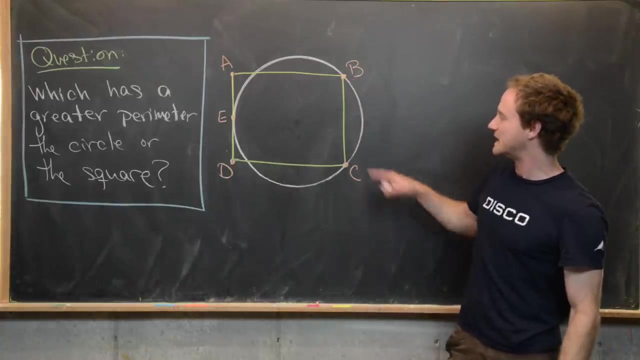 Here we're going to look at a nice little geometry problem. So it has to do with the perimeter of a square versus the perimeter of a circle. So we kind of start with this line, segment AD, and we put that tangent to the circle on this left hand side, And then we find points BC. 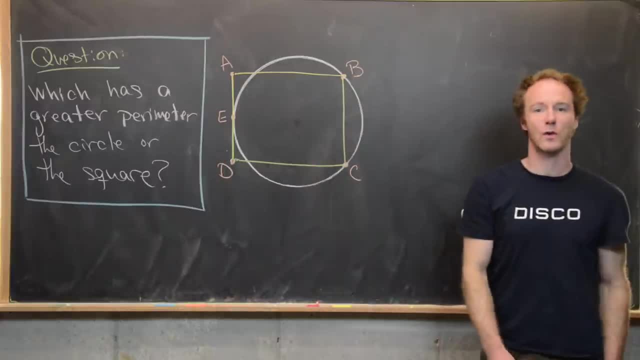 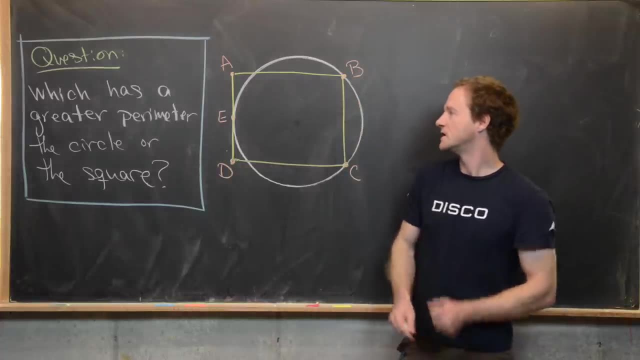 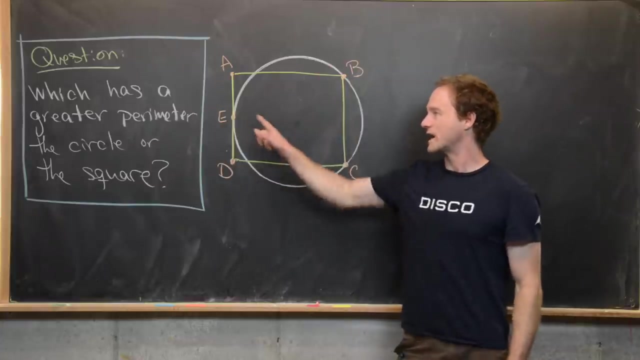 that complete ABCD into a square, And then the question that we want to answer is: which has the greater perimeter, the circle or the square? So in other words, like, if we start at this point, E travel around the yellow versus traveling around the white, which one takes longer. So I'm going to 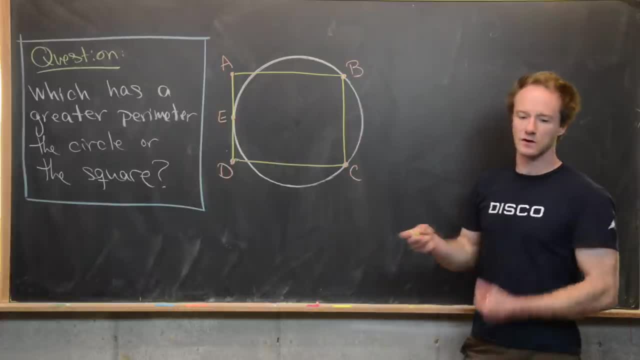 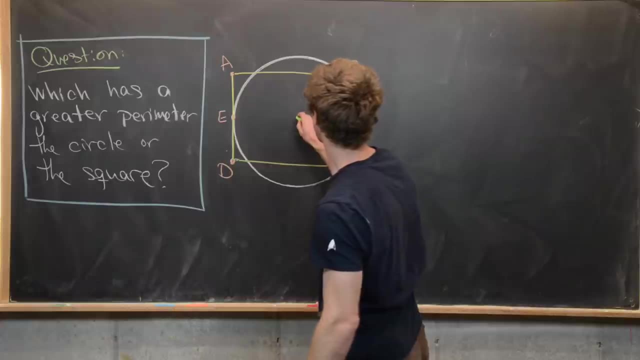 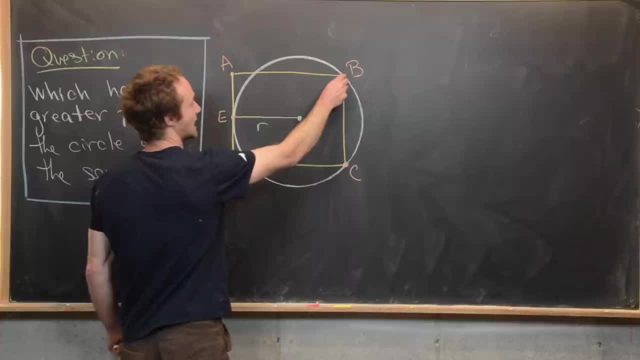 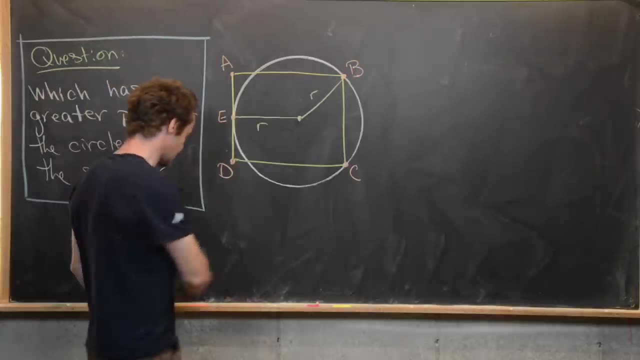 radius out here to E, So that has length R, and a radius up here to B, So that also has length R. But then next we can notice that this length right here, which we could call X, and this length right here, which is something that we could call Y, And then furthermore, we know some stuff, So we know: 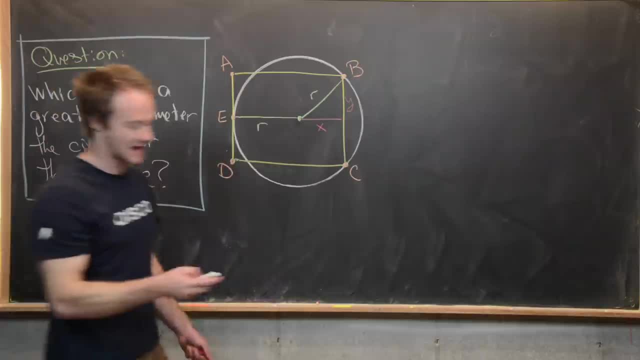 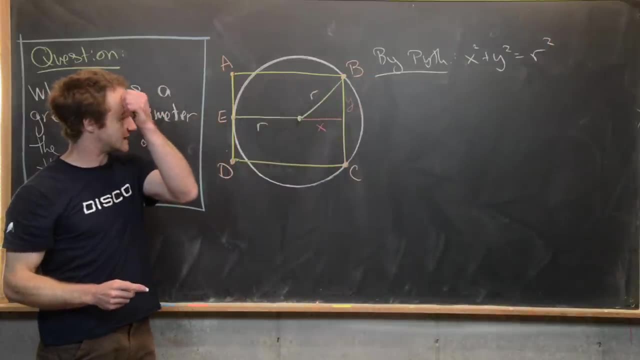 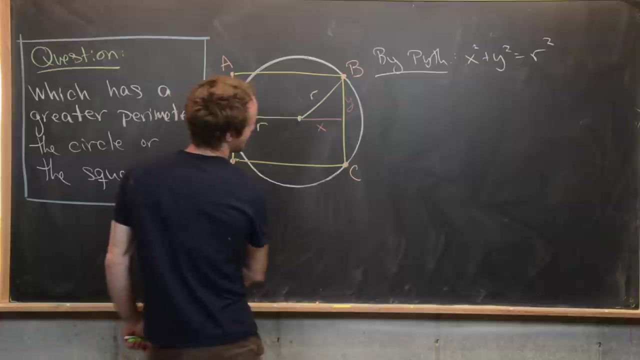 that X squared plus Y squared equals R squared by the Pythagorean theorem. So let's say that Good. And then another thing that we know is the relationship between Y and R and X. So notice that if we put another value of Y down here, we see that the side length of the square is 2Y. 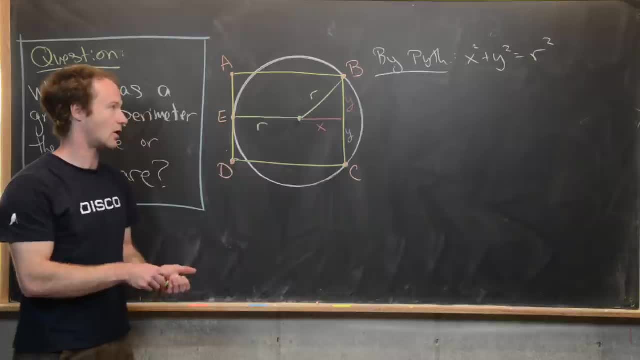 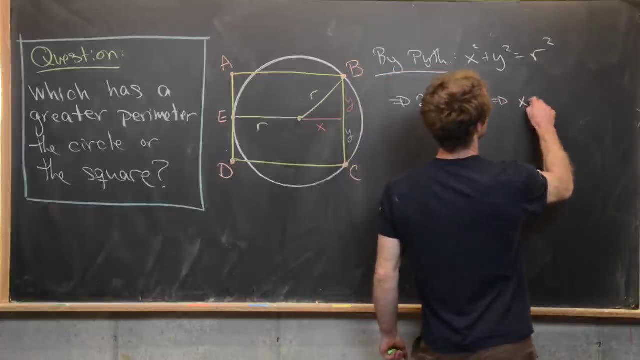 But the side length of the square is also X plus R, So that tells us that 2Y equals X plus R. In other words, X equals 2Y, Y minus R. Okay, so now we're going to go ahead and take this and insert it into this equation. 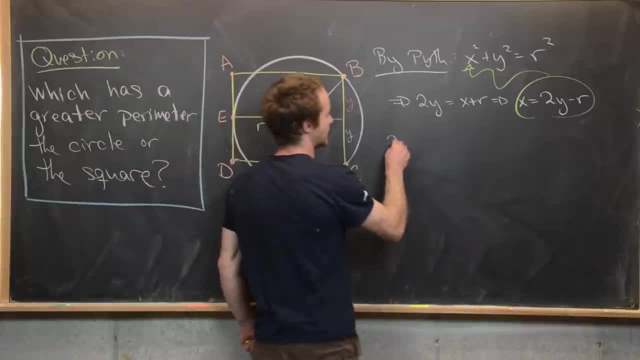 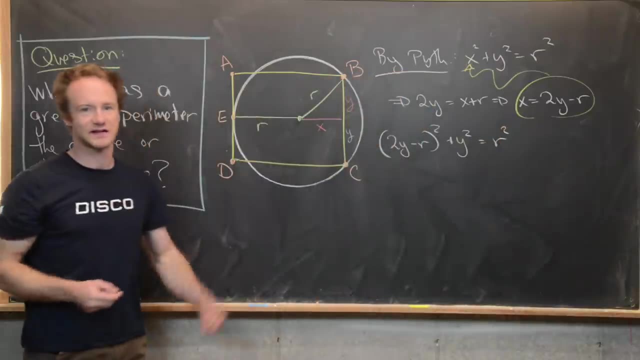 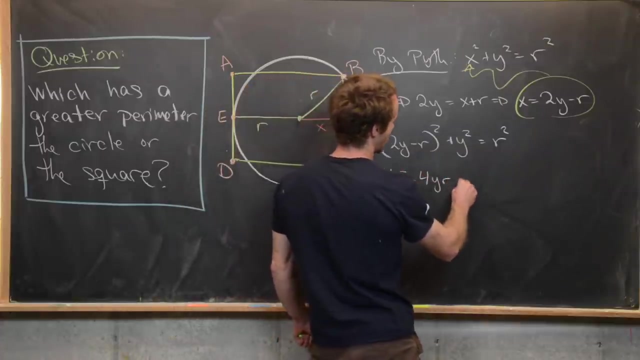 right here. So let's see what that gives us. So we're going to have 2Y minus R, quantity squared plus Y squared, equals R squared. Now, it's just like some symbolic arithmetic, So let's see what we get. We're going to get 4Y squared minus 4YR plus R squared plus Y squared, equals R squared. 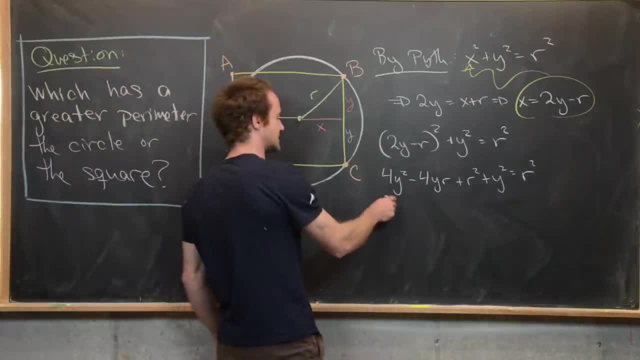 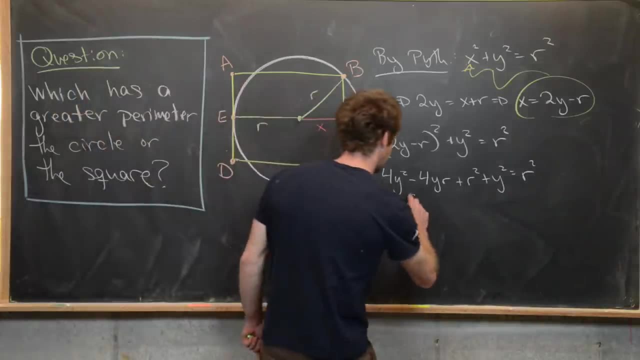 great, but then that's going to give us a nice relationship between y and r, which is exactly what we need. so notice that's going to give us 5y squared. we get that from adding this 4y squared with this y squared and then also notice that the r squareds cancel on both sides of the equation. 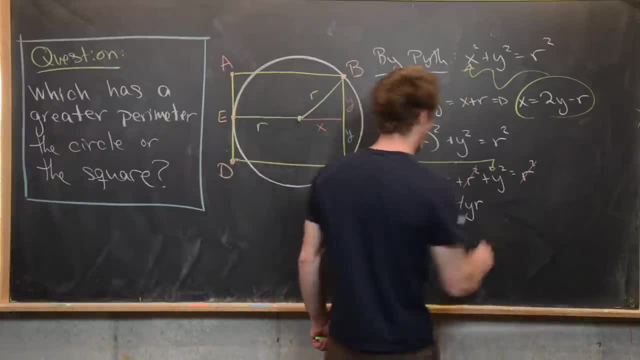 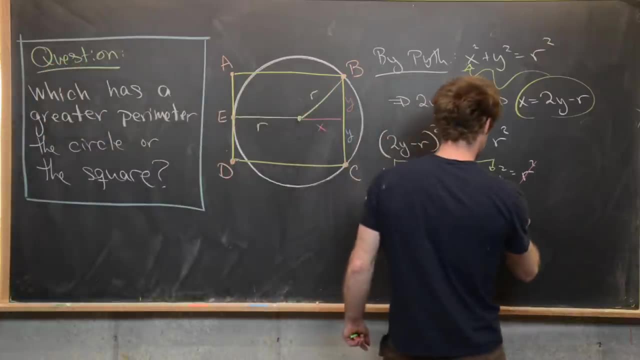 and then we have: this is equal to 4yr. next, we can divide by y, because we know that the side length is not equal to 0, and that's going to tell us that 5y is equal to 4r. so we've got this nice. 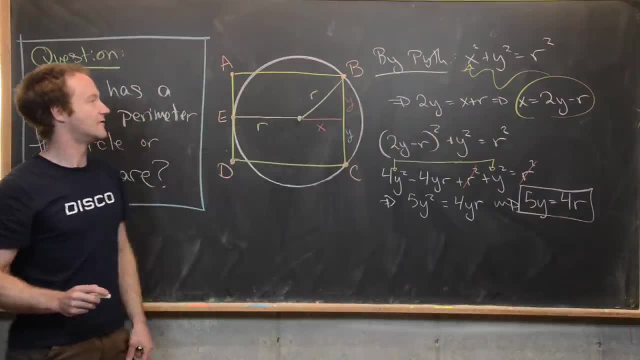 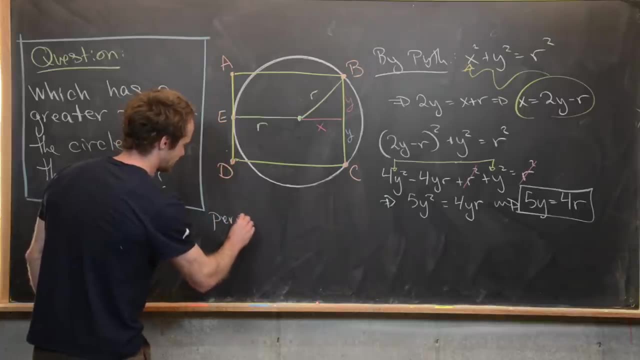 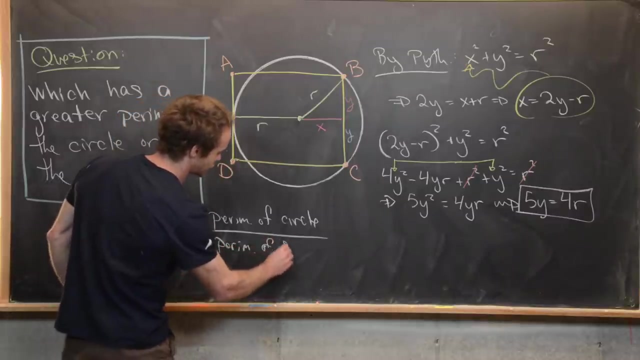 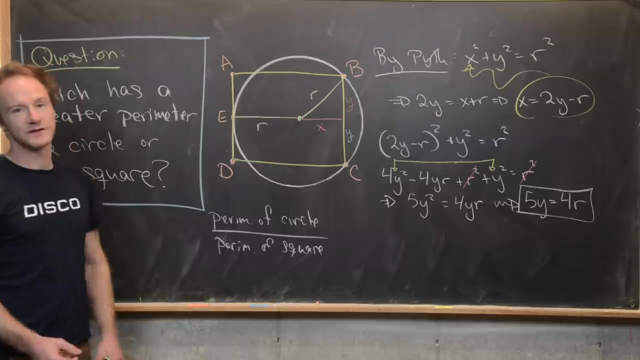 relationship between the side length of the square and the radius of the circle. now what i want to do is look at the perimeter of the circle divided by the perimeter of the square, and if we can show that that is less than one, then clearly the perimeter of the square is larger. but if it's greater than 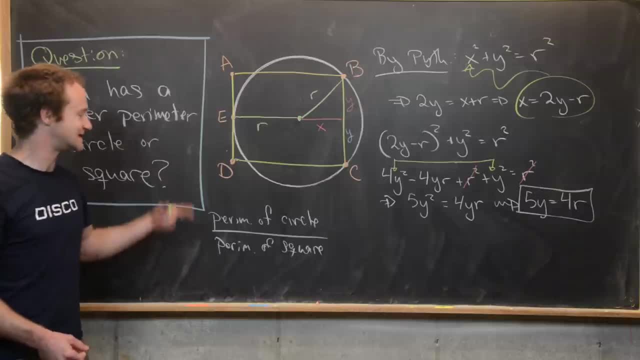 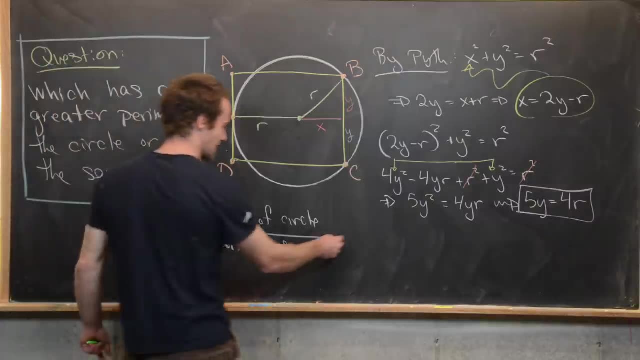 one, then clearly the perimeter of the circle is larger. but it's easier to look at this ratio instead of like doing the calculation without the ratio. so let's go ahead and see what we get for that. so the perimeter of the circle is going to be 2 pi r. you know from the standard formula for: 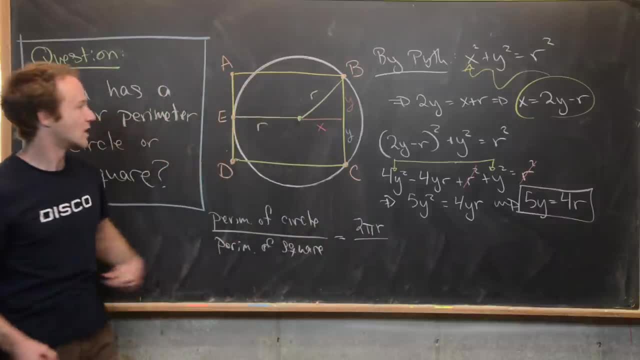 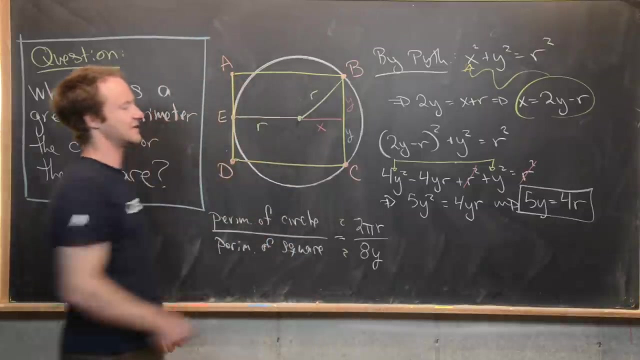 circumference of a circle, then the perimeter of the square will notice. one side has length 2y, so that's going to be 8 y, because we've got four total sides. now the next thing that i'm going to do is take this whole thing and multiply by 2 over 2, so that's going to give me a 4r in the numerator. so here we have 4r times.